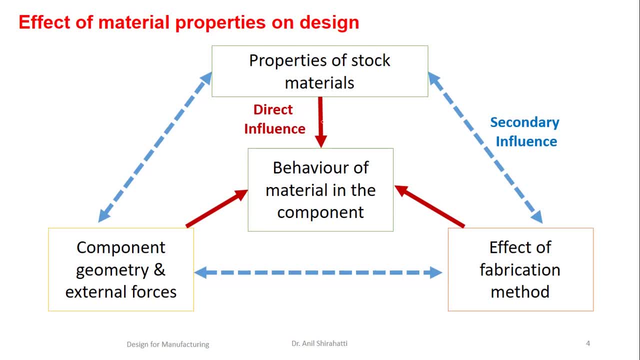 direct influence How it means. For example, if you are creating a stress concentration area in the design itself, what happens? That part will fail early, So that will any component. geometry or external forces will effect directly the material failure, component failure, Definitely when we are having a method of fabrication, for example. 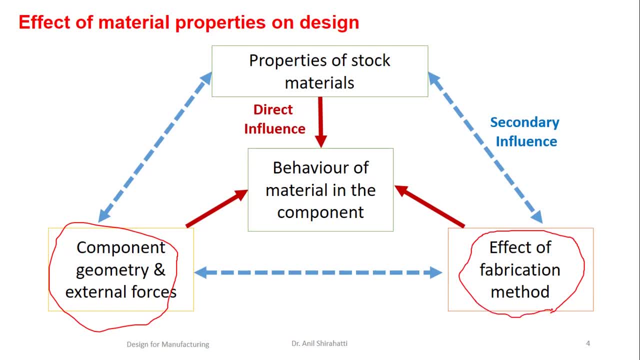 if we are using a welding method for manufacturing, it's strength may be less compared to if you use a single component and do the must in operation, So that will have more strength compared to the welding. So this is why we have a particular method for fabrication. 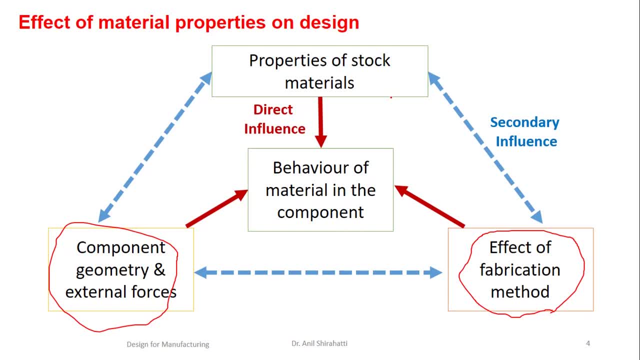 Let's keep going, Let's continue. So if you are using a fabric, let us call it a material. and what about the properties of stock of material? if the parts is very rusted, okay, or it may be have corrosion, corroded part, and if you take that corroded part, okay for manufacturing. definitely. 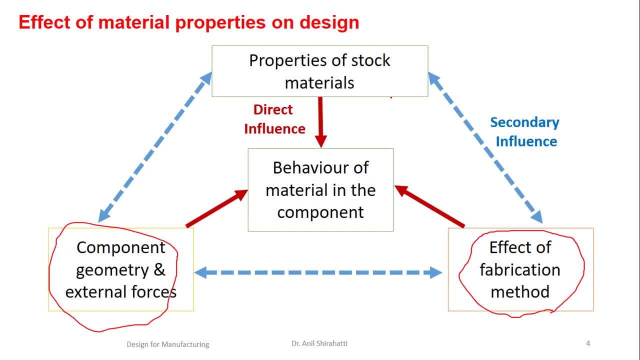 its age will be less okay. so when, suppose, because of the corrosion it has developed some cracks inside the component, and when it goes to the you manufacture the part, and when the components goes to the service, that cracks will elongate, okay, and growth will happen in the material or the. 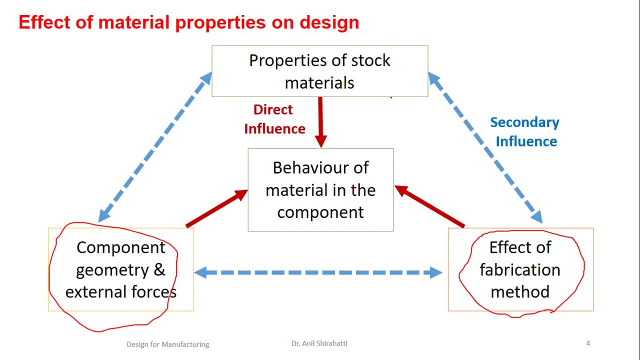 component may fail earlier than the design phase. but if you see the properties of the stock on the fabrication among or component, they are of secondary influence. for example, if I use a stock of the material, for example aluminium or this one is there, let's say stainless steel is there. 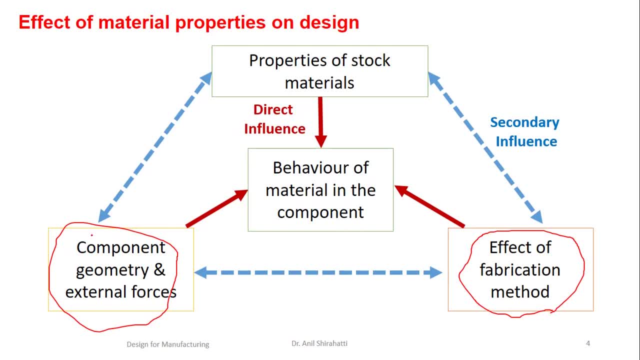 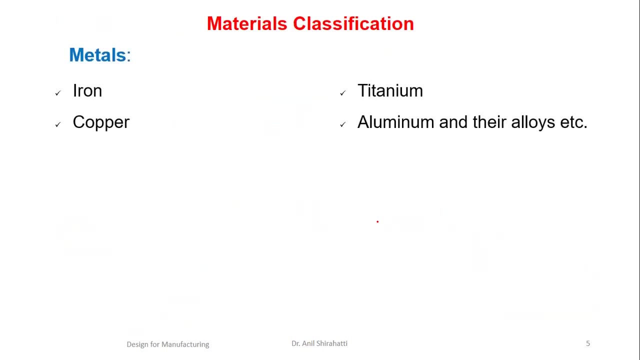 I'll use stainless steel or other materials for. take a further look when I go to the surface, because About their manufacturing on the different types of stress, concentration will not have much effect compared to their influence on the behavior of the material or the components. main How the materials are classified. 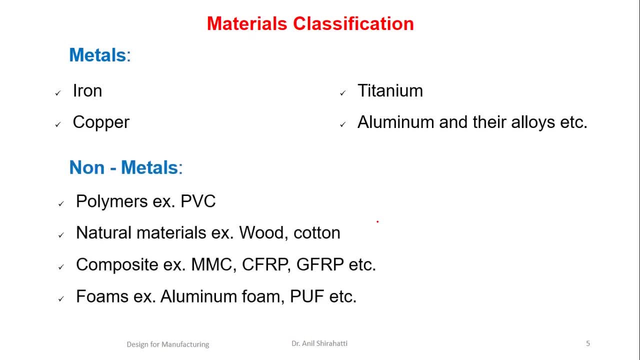 In general materials are classified into two types: a metal and non-metal. So in metal we have iron, copper, titanium, aluminum, etc. Non-metal will have composites. We have foams, which are new type of material, Then natural material like wood and cotton, or polymers like PVC. 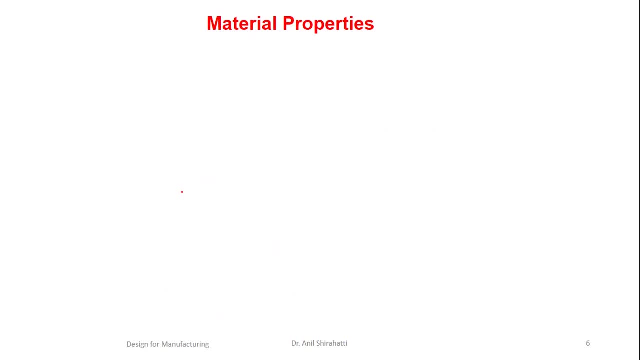 Also, whenever we are designing any material, the marketing properties place an important role. So, as a designer, we should have a clear idea about what are the properties of material which we are choosing to make that component or make that assembly. So what are the parameters or properties? we will check. 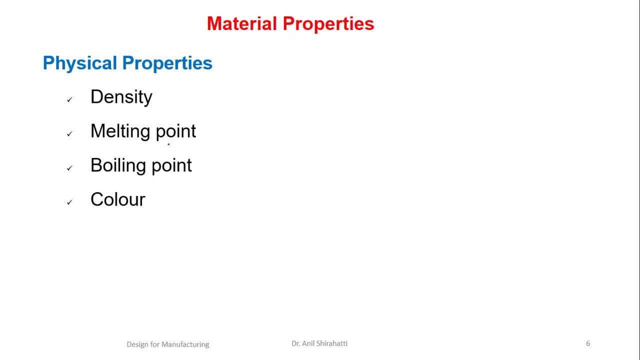 There are the physical properties, For example Density, melting point, boiling point, color. Now, if the weight is the main concern, then the density plays an important role while selecting the material. Suppose the load is not much, but we want a material with less weight. 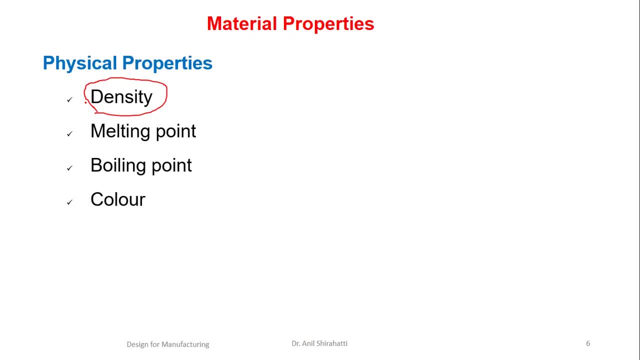 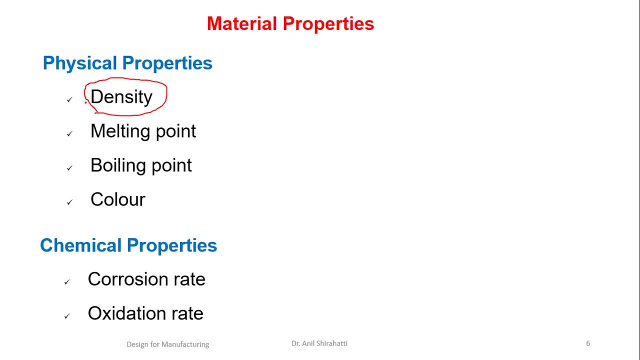 So these are the properties of the material. So these are the properties of the material: Coefficient, intense, tetra, confident, as you can see. And then if we are using any material in sea or sea type environment or corrosion type environment, We may have to go for stainless steel. 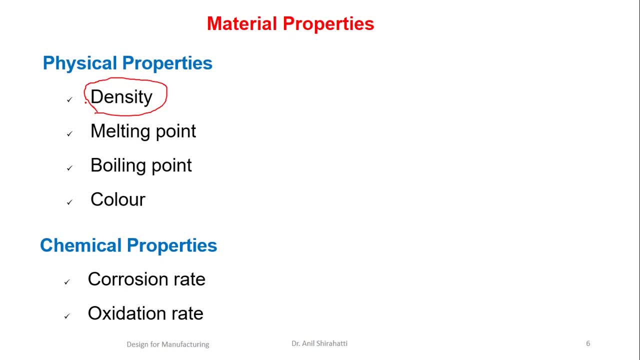 We may not go for mild steel components Or mild steel as a material. Then the thermal conductivity, Like thermal properties, like conductivity, specific heat coefficient of expansion, fire resistance of that material. So definitely where the fire is there I cannot go for plastic or any polymer. 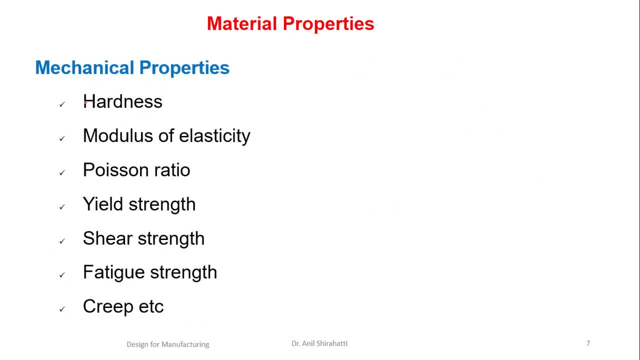 I have to go metal. Okay. Next are the mainly what we are concerned. in much of the designs we will see the this properties, that the mechanical properties like hardness, modulus of elasticity, Young's modulus, Poisson's ratio, shear strength. so all this yield strength, shear strength, everything. 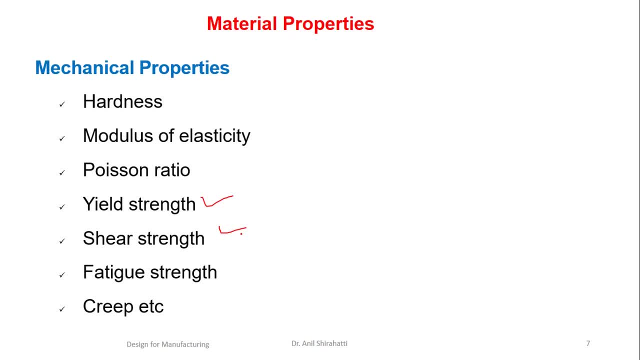 we can calculate using: if I do a test of tensile test, then if I do a fatigue test, I can find the fatigue and grip. it is with respect to temperature either. it can be done at high temperature, also at room temperature. so creep is nothing but the behavior of the material. 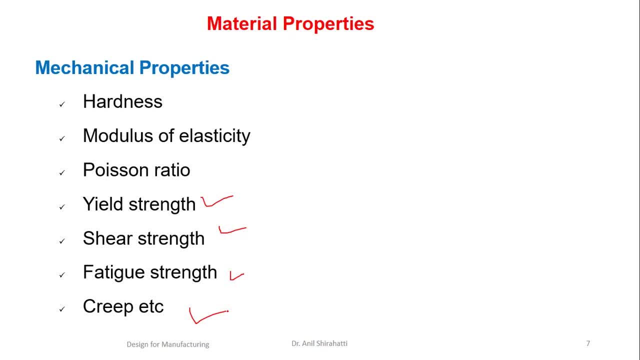 with respect to time either. generally, the creep is very serious matter if it is at high temperature, like nuclear power plants, where the material will be working at 550 degrees centigrade- in some cases it go till 650 degrees centigrade- then the what are the fabrication? 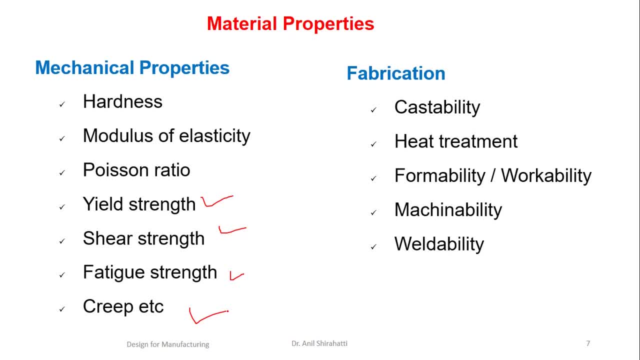 method of manufacturing method you are adopting, like castability, heat transfer. If you are doing what, the changes may happen because of the heat treatment. if you are using a welding method to definitely the parts, the component which is welded, the position of welding, wherever you are doing near to that, there will be change in the property. 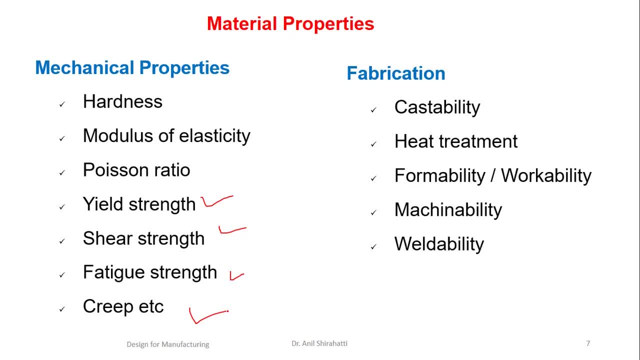 of the material, okay, and if the material is machinable or not. suppose I choose a material which is mnemonic and I want to reduce its diameter from 100 to 50. it is very difficult, you cannot machine it very easily, but if you go for milestone, definitely you can take one mm to mm depth of cut and 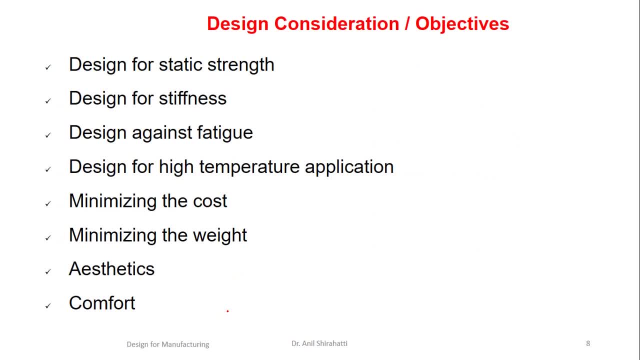 reduces. next is: what are the design? as a designer, you will consider different consideration while designing the any product. one is the static strength, then the stiffness of the material, also against the fatigue of I am designing. if I am designing against a high temperature application, I have to see the creep properties. overall, my objective will 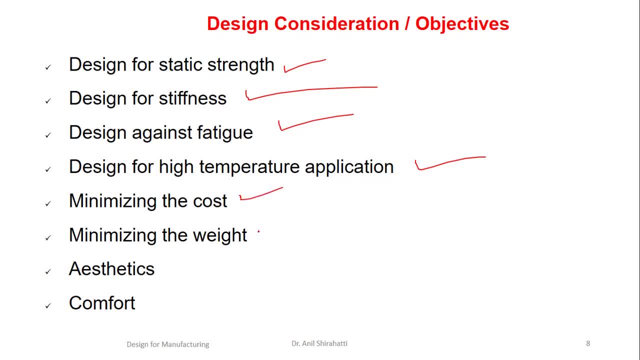 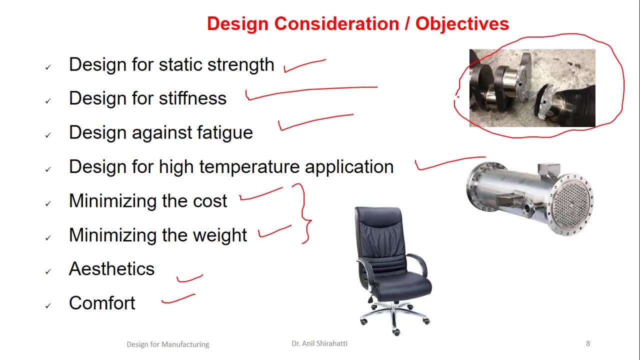 be. in general, any designer should be: minimize the cost, minimize the weight- okay, that is also important and in some cases, aesthetic and comfort and so place an important role. for example, if I see this part which is nothing but a crankshaft, where the major concern is the fatigue properties, 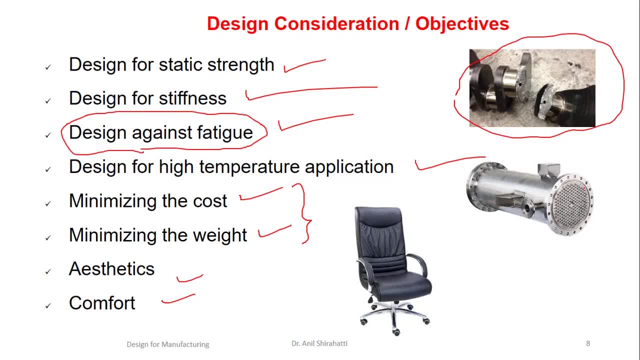 so the design from the fatigue point of view is important, but if I am doing a heat exchanger, the main concern is a high temperature application. Okay Now next, if you consider the from the chair point of view, is it should be aesthetically good enough? definitely, it should provide a comfort because a person will be sitting on. 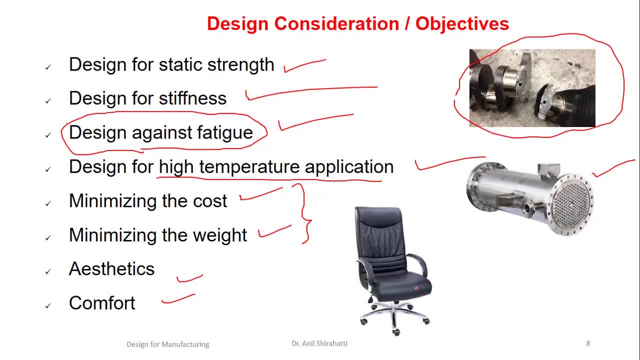 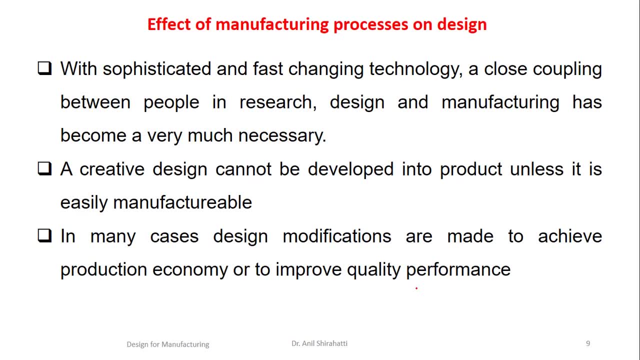 the chair for continuously, maybe for eight hours, so you should comfortably sit in that chair very easily. next up, there are a few effects of manufacturing process on the design. okay, with a sophisticated and fast change in the technology, a close coupling between a people in design- Okay. 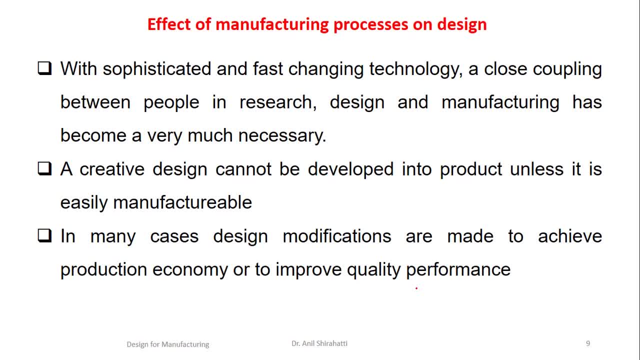 So the research design in manufacturing has become very much as essential, necessary in today's world. a creative design cannot be developed into a product unless it can be easily manufactured. so you cannot develop a good product if you don't have an idea about the manufacturing. in many cases design modifications are made to achieve the production economically. 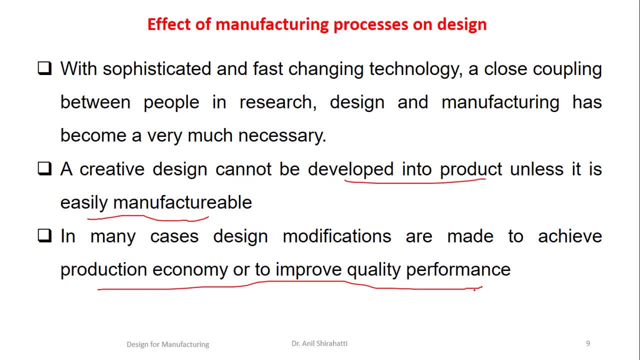 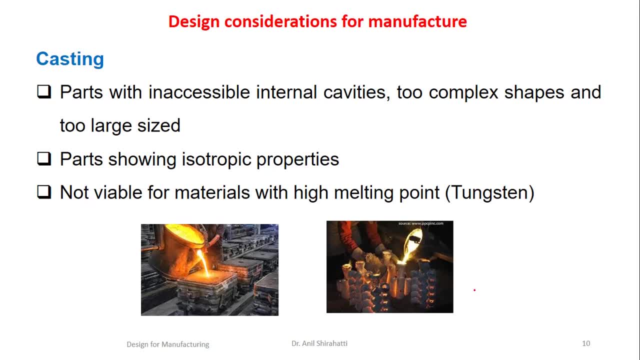 and improve the quality performance. now, for example, what are the design considerations? Okay, Okay, Okay, Okay. So, for example, when I am doing a heat exchanger, I don't have the right material for the machine, So I am going to see the materials for the heat exchanger. option is actually, if I am doing 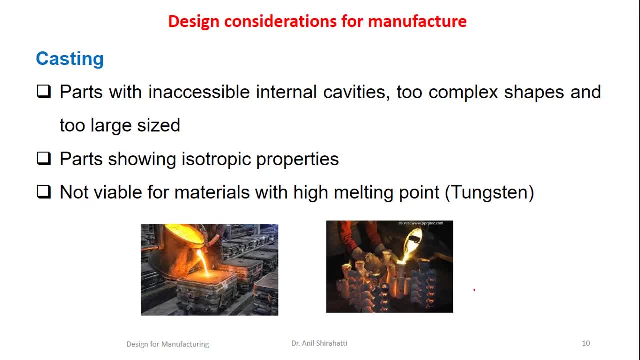 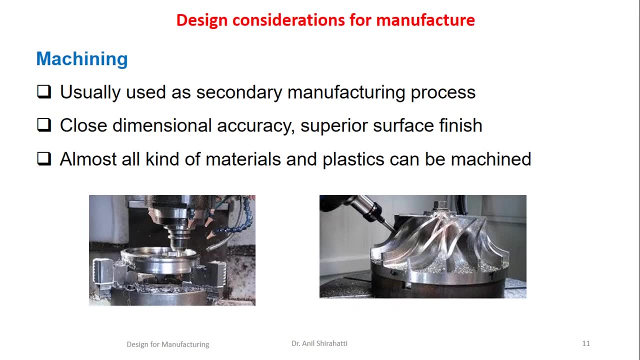 for a tungsten material not viable for material for high melting point. Definitely tungsten will have very high melting temperature so I cannot go for casting so easily When I am doing any casting operation. design parts with an accessible internal cavity from complex shapes or too large size should be avoided. 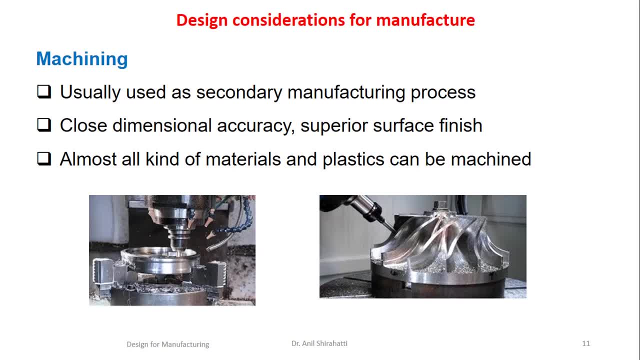 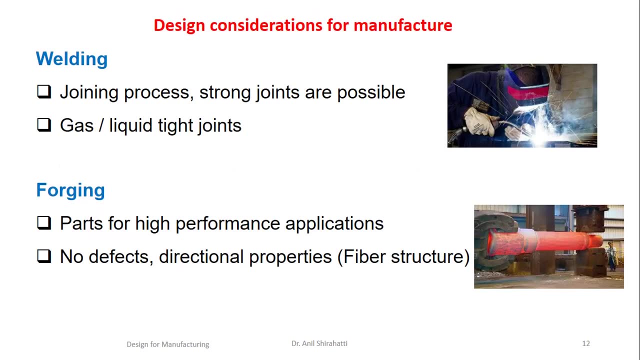 Okay, manufacturing process: close dimensional accuracy of maybe 100 micron or less than that is possible in case of a machine. it depends upon the machine and the process of machine you are using. almost all kind of material or plastic also can be machined. if you are welding, you are using welding. 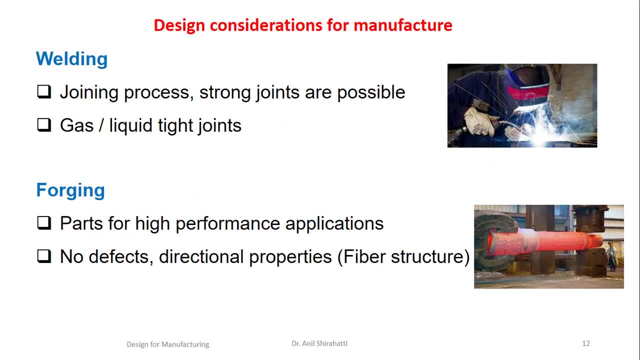 operation. it is nothing but joining process. strong joint is possible. you can have different arc welding, gas welding. different depends upon the application. you can choose the welding process. if you are going for forging, parts of high performance applications are manufactured using forging, no defects and directional properties like fiber structure. next, if you 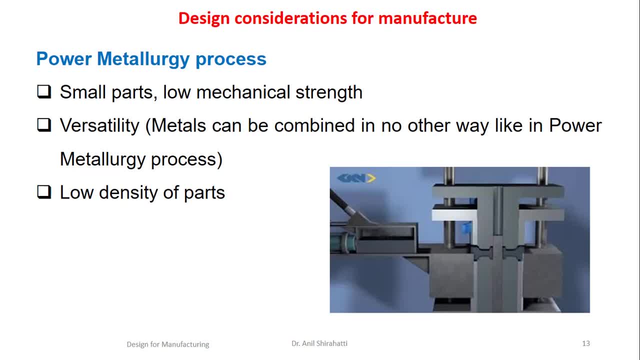 are using a powder metal is like mixing of two metals you want. it's better to go for powder metal. engine with a low density parts can be made, but the only thing is the initial investment in this process is very high. so always recommend it for a high, high number of. 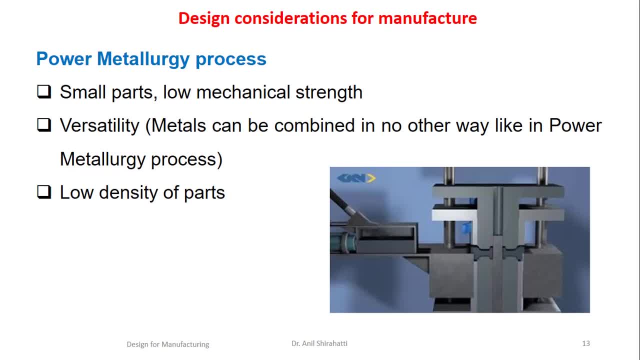 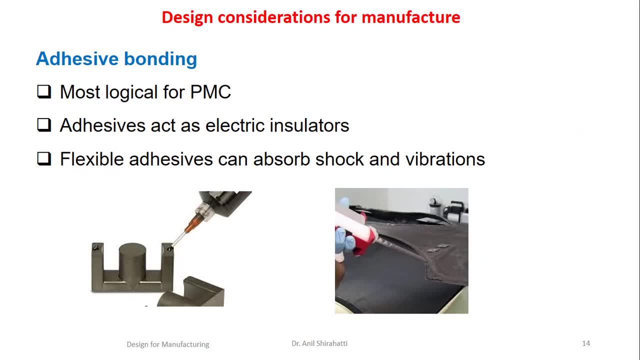 oil and gas applications, if you are going for forging parts of high performance applications, or if, if the production quantity is very high, you can go for powder metal process. adhesive process is a general where here the strength is very less, but it is good when you when there is. 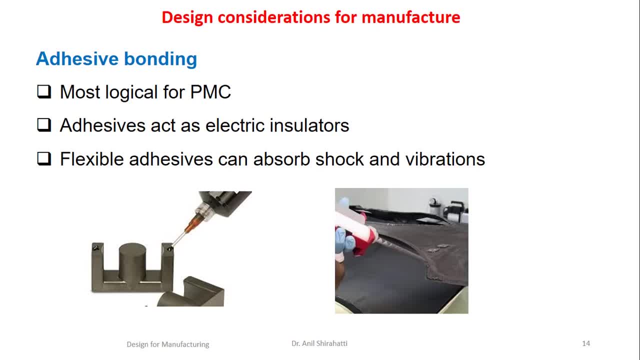 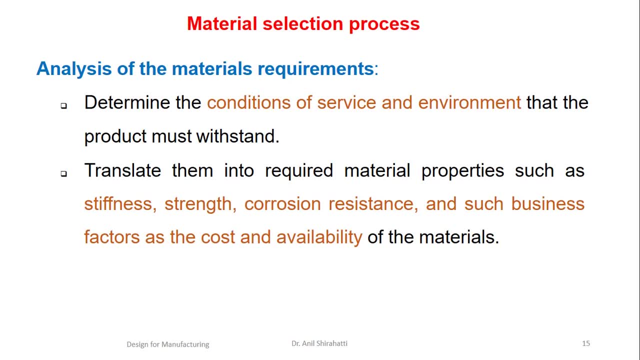 any electrical insulators or flexible adhesive can absorb also shocks and vibration. these are mainly used for PMC components. now what about the material selections? okay, now let's analyze for the material requirement. the first you have to do it determine the condition of service and environment that the product should withstand. you have designed. 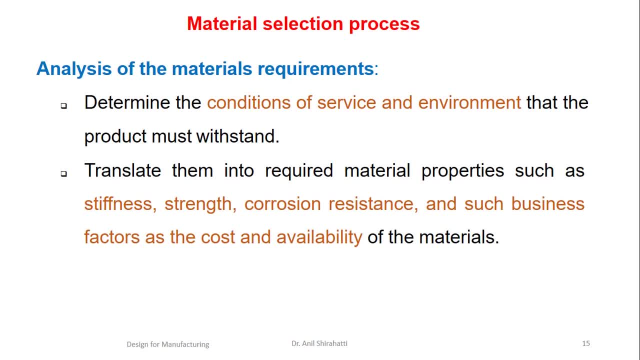 everything, but what is it's working or environment condition you have to check now. this may be: what is the stiffness strength if the environment is corrosive in nature and so the business factor like cost and availability of that material very easily and place an important role while selecting. 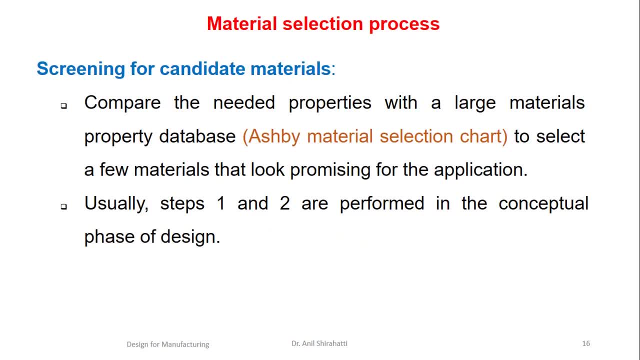 the material. second is you can use a material that has a very high cost and availability of that material very easily and place an important role while selecting the material. second is you can use a SBA material chart for the material selection. okay, you may have given the different options, so 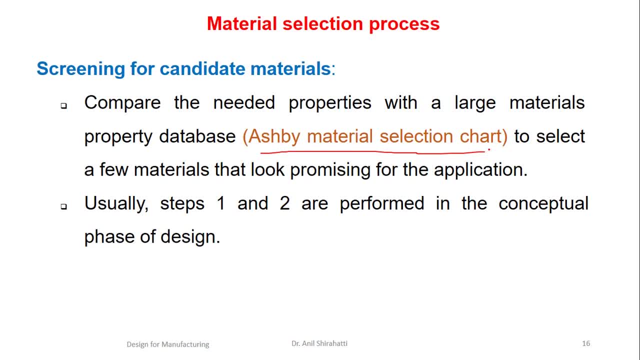 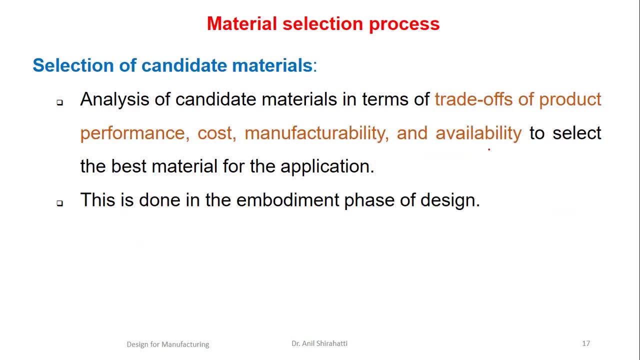 you can add your variables, like properties. next you can add the cost, availability and then do the selection. so this chart will help you in that part. okay, so the more detail about SBA we will see in the last few slides. and so selection of candidate material. so first steps. what you did was 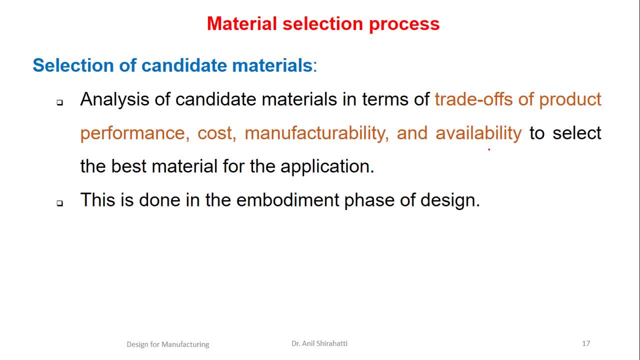 you have depends upon its technical details, cost, availability. you have selected few parts. then, using the SBA chart, we have found like three to four parts which can fit your technical details. and so, whatever the environment details everything face, then you have to analyze this on terms of. 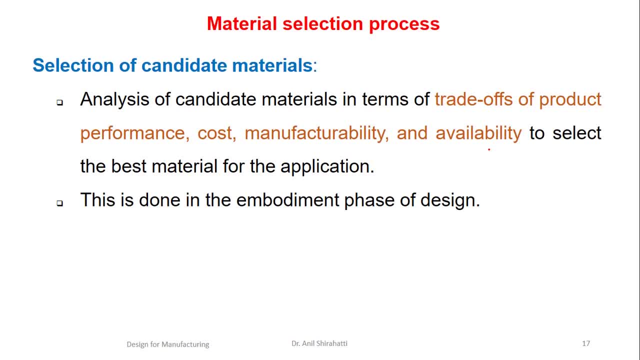 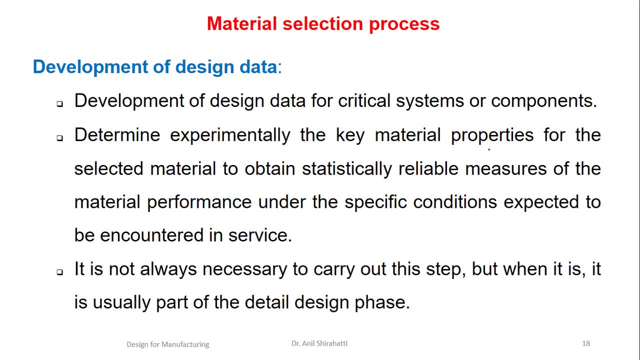 performance, cost, manufacturability and availability. so to select the best material among this different materials or options given, then you go for the more detailed development of this design. so development of design for a critical system or component: determine experimentally the key properties, material properties for selected. 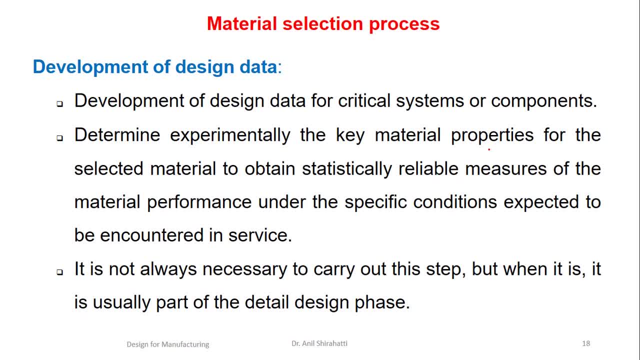 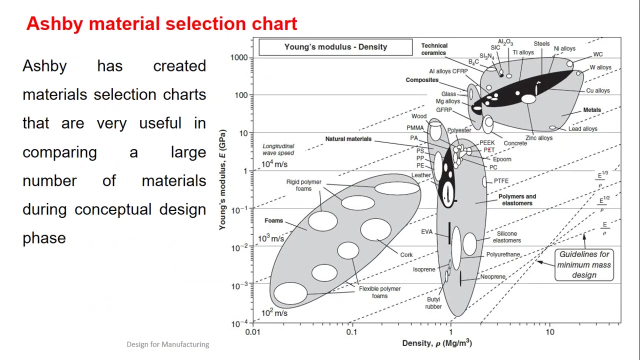 materials to obtain statically reliable measure of material performance under the specific condition expected to be encountered in service. it is not always necessary to carry out this step, but it is useful part of detailed design. what it says is N, N, A, N, K, P, L, T, T, T. 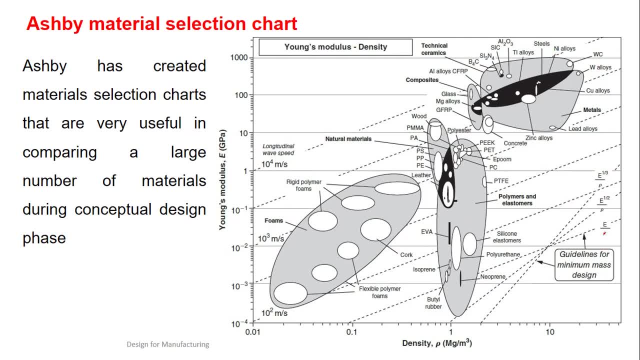 Z, young's modulus. okay, now, whatever the curve you are seeing, let's say this curve is e by, that is young's modulus by density. this curve is young's modulus by, raised to square root of young's modulus by density. like this, few curves are there. now let's say i am interested in some x or y. 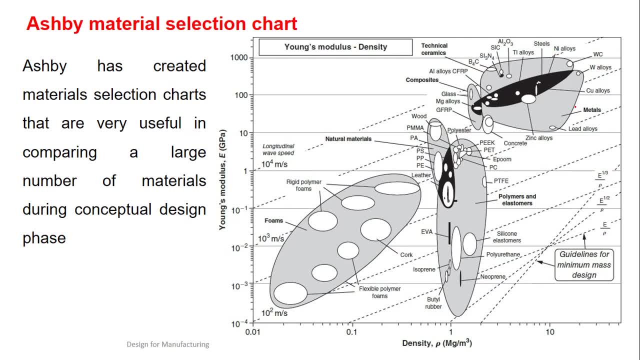 material. so what i do is i will do all my technical calculation and i get a ratio of e by p, so e by density. so e is nothing but young's modulus, that is, the material properties. d is not, rho is nothing but the density, so depends upon that i can get a ratio. so let's. 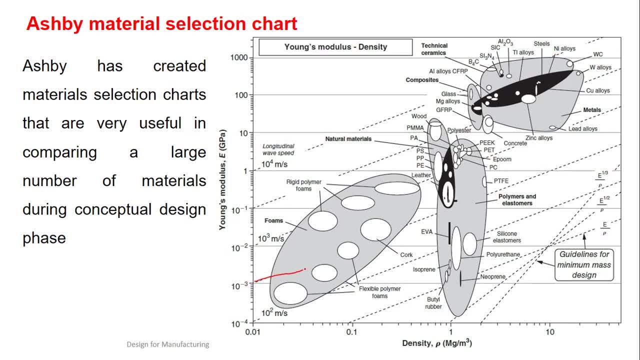 see that ratio is some somewhere between 10 to minus 3, so i will get this curve okay. so this line is defined by, let's say, e, by rho. that is density. now, if you see from this chart anything acting above this one, i can select anything. 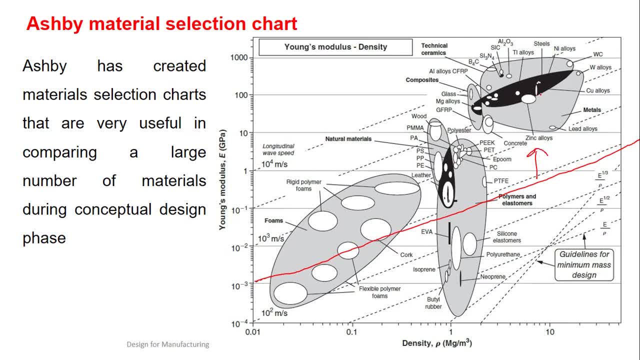 material. so what are the material available? so i i can select steel, i can select titanium, i can select composite, i can select natural fibers, i can select few foams also. now this first i have given i got a lot of options of selecting the material which is technically satisfying my 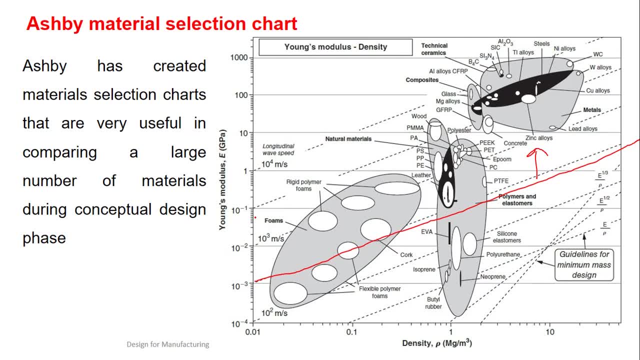 design needs. now next phase is: what is the availability of that material? so let's say, foams may not be easily available, so i can say, okay, i don't want that one. now i have option of: wood is easily available, steel is available, titanium, all these are available. so now what about the cost? then i i may go and select steel because i saw 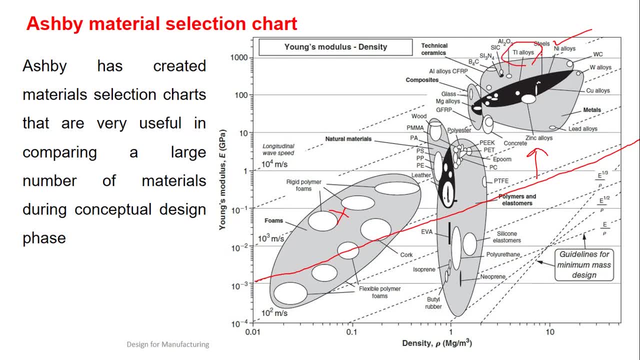 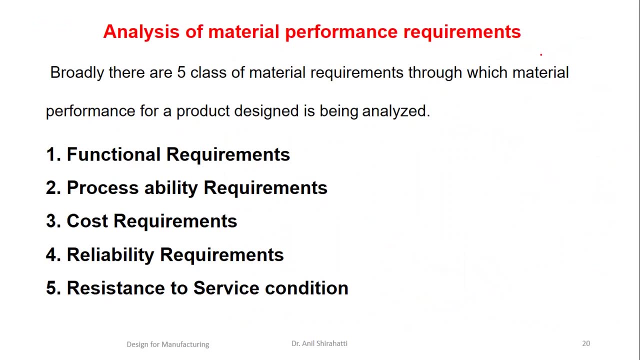 that titanium is very costly. still, both are satisfying the needs, but still is more cheaper compared to that one. so like this, you can select the material, decide. the final material depends upon the whatever the alternative materials available for you. now the last part is analysis of material performance requirement. so broadly there are five. 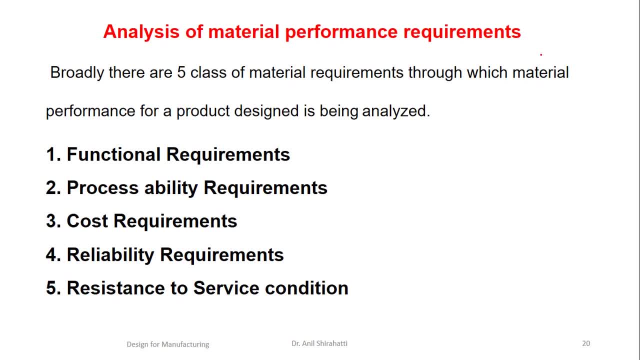 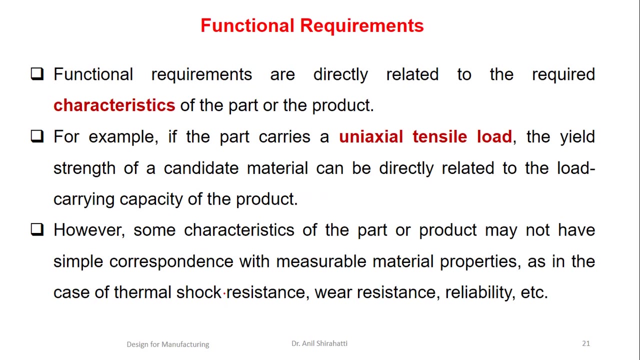 class of material requirement through which the material performance for a product design is being analyzed. first is the functional requirement, next is the process of processability requirement, cost requirement, reliability requirement and resistance to service requirement. so we will see all this in a brief, so let's start with the first, that is a functional requirement. so functional requirements are directly. 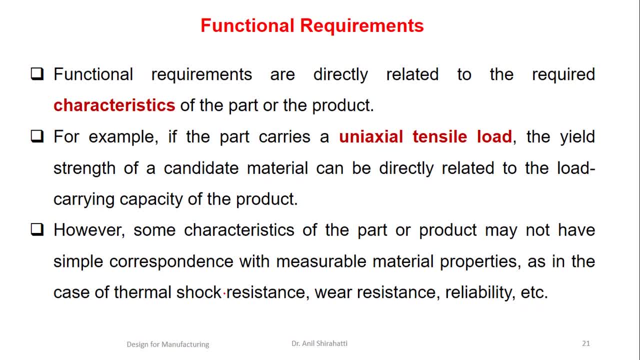 related to the required characteristic of the part or the product. for example, if the part carries the uniaxial tensile load, the main thing, what? what is the yield strength of that material can be directly related to the load carrying capacity. okay. however, some characteristics of the part or product may 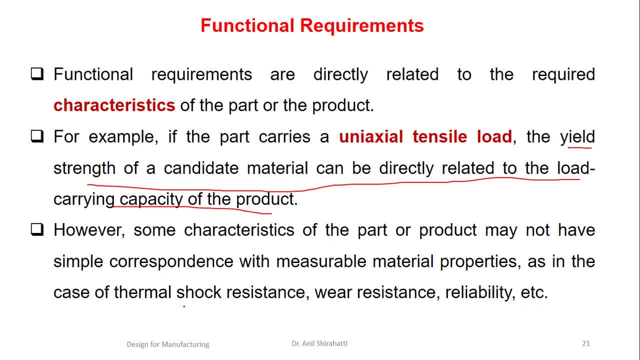 not have simple correspondence with the measurable material property. as you can see in the video, i am in case of a thermal shock, wear resistance, okay, reliability, etc. so in these cases, uh, if there is a thermal shock and wear resistance needed, so i may have to uh connect the wear test performed on that. 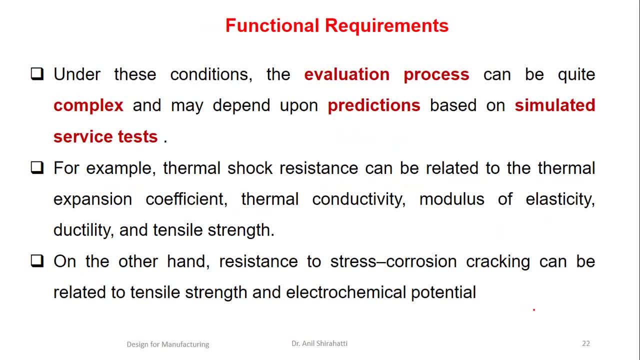 material to the wear rate. okay, under this condition, evaluation process has to be done. for example, what i said was: if, if i i am concerned about the wearing of the material, i have to do the wear test and check what is the wear rate with respect to the wear test and check what is the wear rate with respect to the 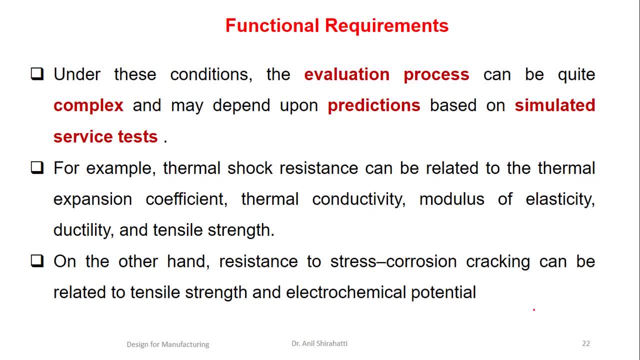 load acting, which also with respect to the distance, all this parameter i can decide and then decide the material. for example, in case of a thermal shock, i have to link the thermal shock resistance to the thermal conductivity and the expansion coefficient of the material. okay, definitely in. uh, in some cases if the resistance of stress, corrosion, cracking, 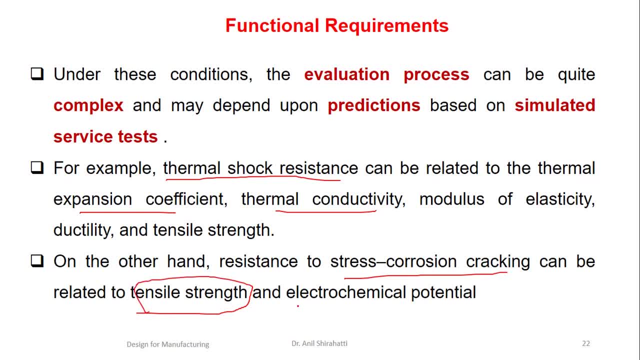 can be related to the tensile strength under electrochemical potential, so i can create a corrosion type of environment okay at the laboratory level. so for example, uh let's assume a ship, so ship impeller. so what happens to the ship impeller? it is uh inside the sea which is a. 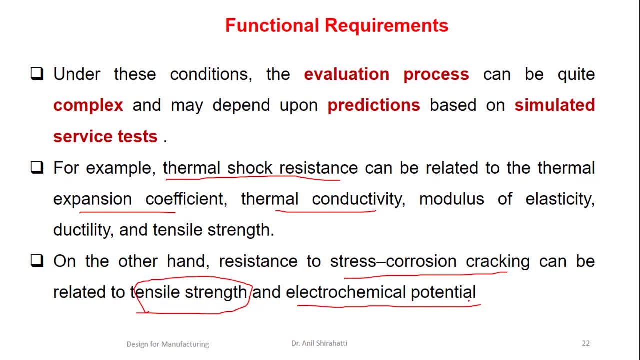 corroding environment. so maybe after a few months or few years it may start corroding. but when i am selecting any material, i cannot wait for, let's say, two years and decide one material. so what i do is i will make, create an electrochemical potential, electrochemical environment in which the corrosion rate can happen within five days. the 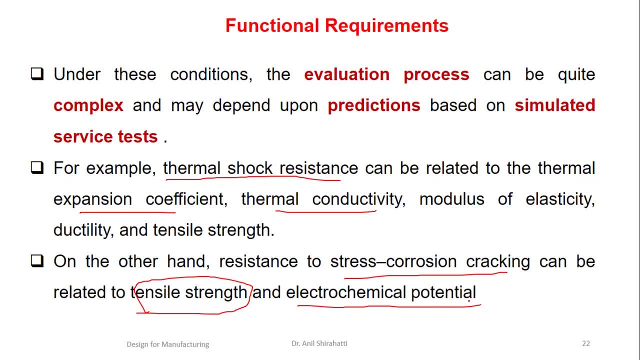 material can corroded. equivalent to the material can be corroded after five years in actual working condition. so let's say i am using stainless steel as a material, okay, and that may get corroded after five years by, let's say, by five percent. so the same scenario of that material can be created in. 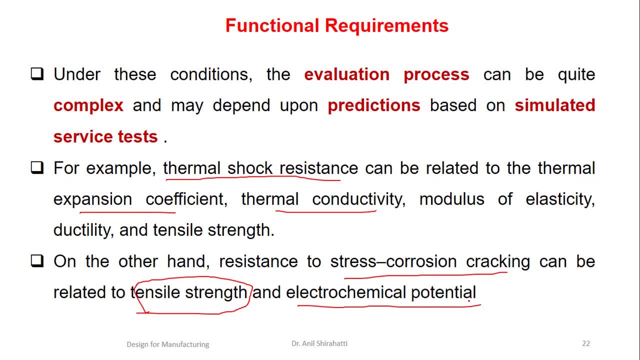 the laboratory in a corrosion environment, chemically corroded environment, which the same environment or amount of corrosion can be created in five days. so this is called accelerated corrosion. okay, there are standards, a stream standards, to do that, and then i can decide whether i have to go for stainless steel 316, 304 or whatever part. 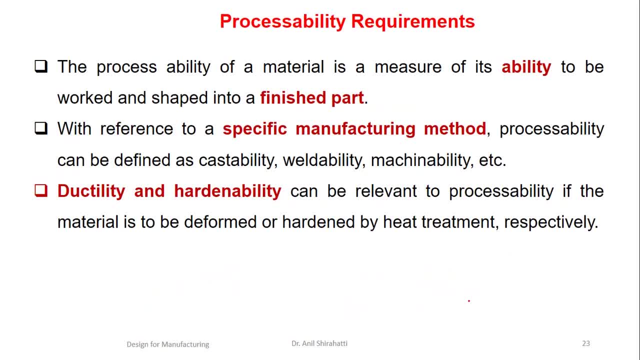 next is a process ability of requirement. okay, so process ability of a material is the measure of ability to be worked and shaped into a finished part. with reference to specifically manufacturing method, processability can be defined as: in case of a casting, castability in case of welding. weldability in case of a machining process. 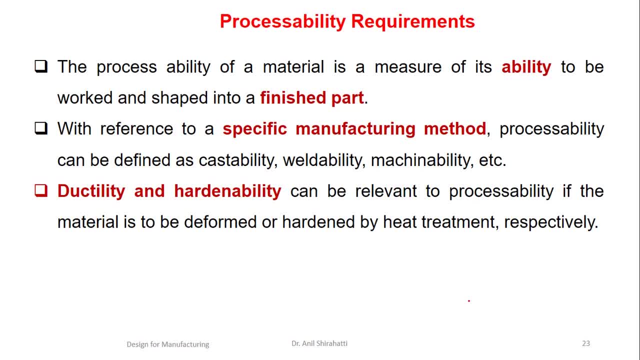 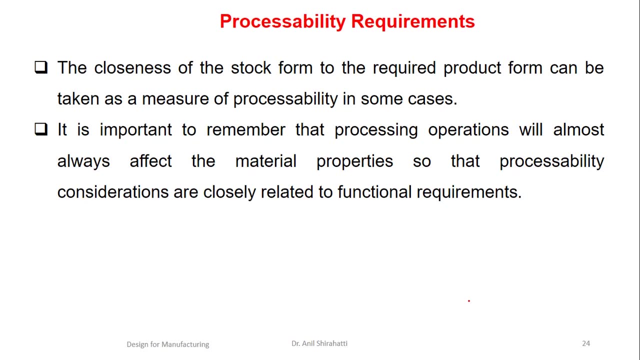 machinability etc. so ductility and hardenability can be really relevant to the processability if the material to be deformed or hardness by heat treatment process, the closeness of the stock form to the required product form can be taken as a measure of processability. in some cases it is. 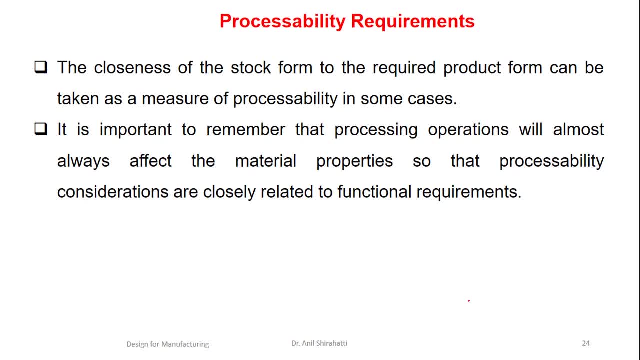 important to remember that processing operation will almost always affect the material properties, so that processability consideration are closely related to the functional requirement of any part. what I'm going to say in processability- suppose you don't want the material properties should change very heavily. you should go for a machining operation compared to a welding. 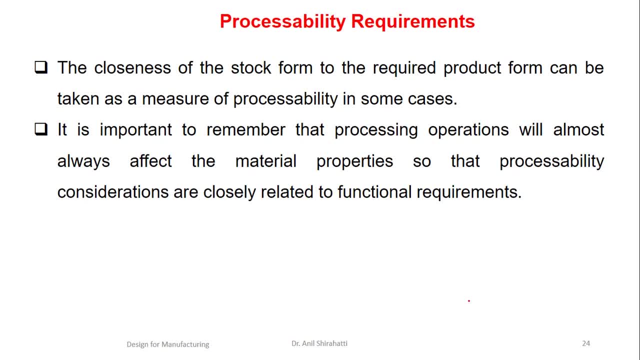 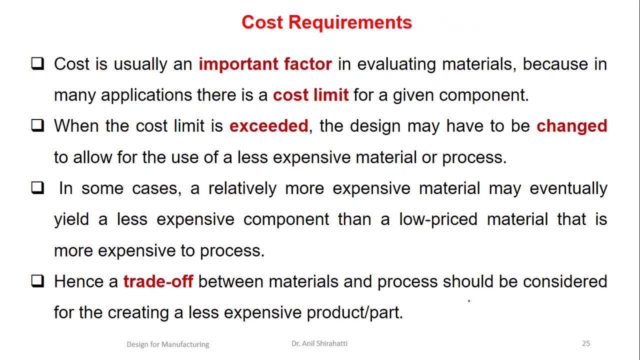 operation. okay, because definitely when you are doing a welding operation near to the weld, huge amount of heat treatment, heating happens and the material property at microstructure level will be changed very heavily cost. so cost is also a very important parameter when we are taking the design or selection of a. 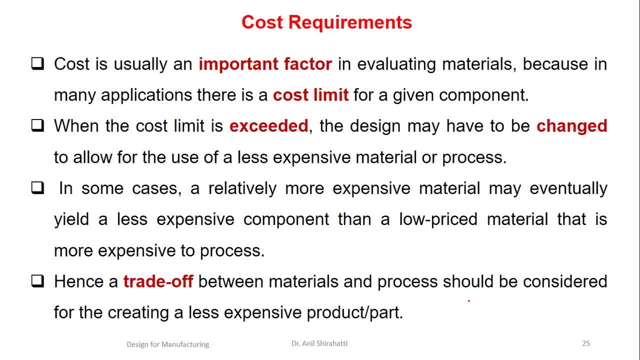 material in the design phase. so cost is usually an important factor in evaluating the material, because in many application there is a cost limit for a given component. when the cost limit exists, the design may have to be changed to allow the use of less expensive material of the process. 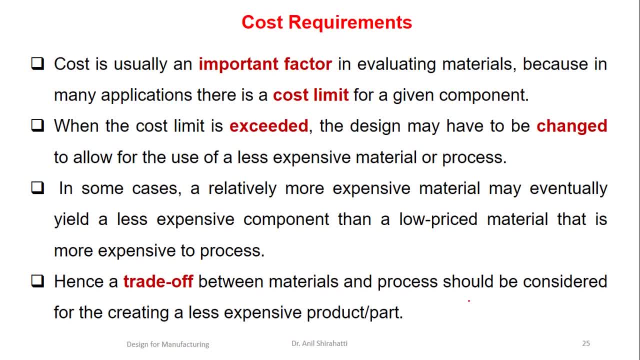 in some cases, a relatively more expensive material may eventually yield a less expensive component than a low-priced material that is more expensive to process. hence a trade-off between the material process should be considered for creating a less expensive product. so what it means is, in some cases, suppose 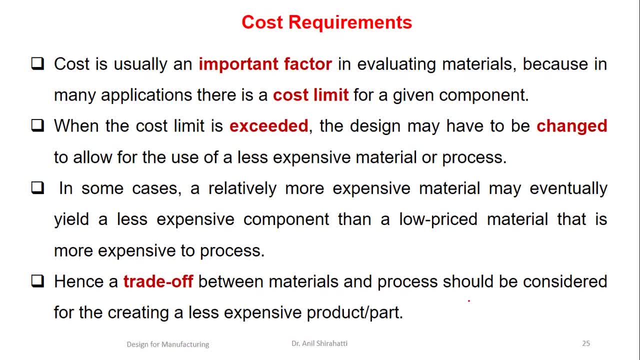 I'm going for a selection of material. okay, the material is going under some tensile load, so I can select a mild steel also. and let's say I got a yield strength of whatever the load acting is having a yielding of. maybe let's say 100 mega Pascal, 150 mega Pascal. so for 150 mega 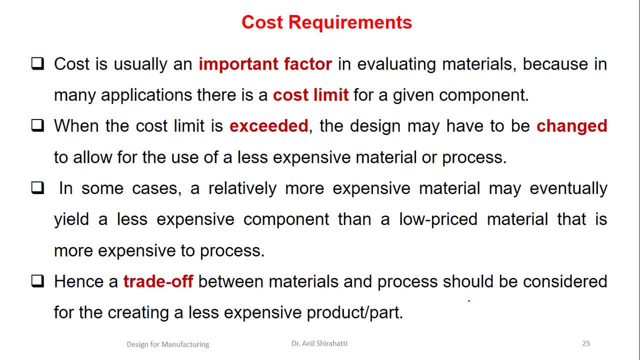 Pascal of load I can easily select, let's say, mild steel, which can work, or even I can select stainless steel. but if I see the cost wise, the mild steel will be around 55 to 60 rupees kg, but definitely stainless steel will be about 300 to 350 rupees kg. so there the cost place an. 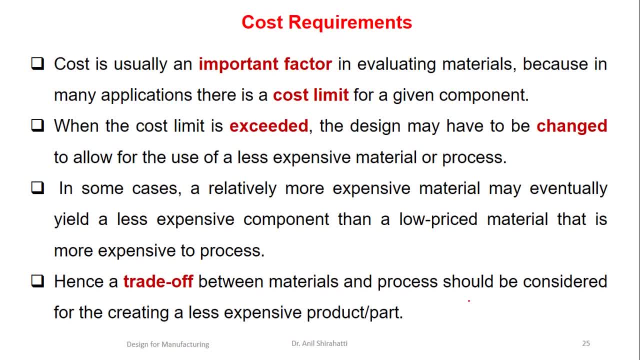 important role. but if the same material I'm designing for, let's say, for high temperature application- okay, let's say I am working for 300 or 350 degree centigrade, where it is a very critical nuclear operation, okay, some nuclear component it is going, in that case it is better to go for. 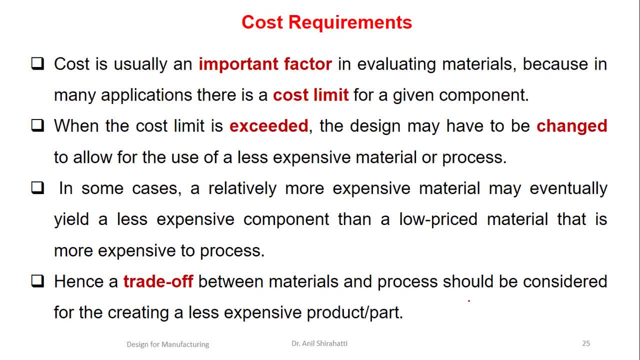 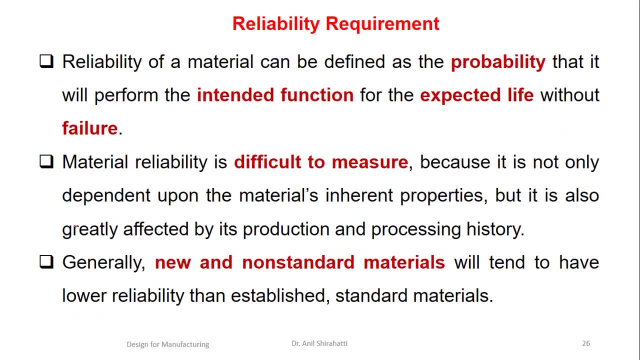 stainless steel, because the amount of risk involved is more than the material cost. so that is what I am saying in this third point. next is the reliability of the requirement. so reliability of the material can be defined as the probability that it will perform the intended function for expected life. 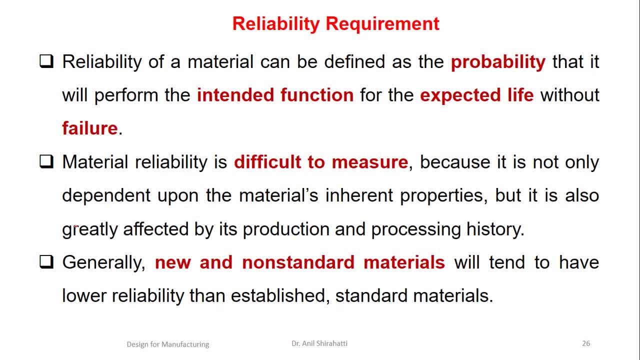 without failure. so what I explained in the last example, so definitely both can be defined. so that is why a temperature of 300 degree or to 350, but definitely with respect to the time, the stainless steel component will be having better life compared to a mild steel component. material radiability is difficult to. 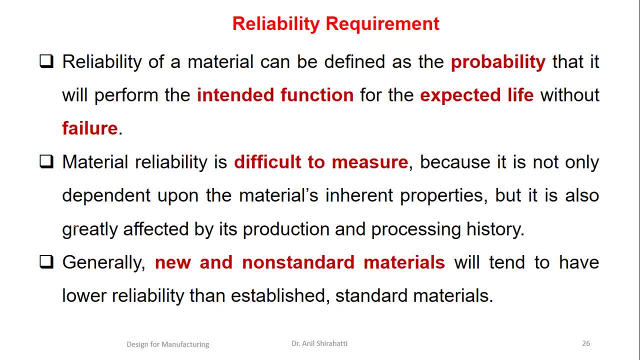 measure because it is not only depend upon the material inherent property but it also greatly affected by its production and process history. generally, new and non-standard materials will tend to have low reliability, and so the reliability. then they establish a standard materials that also, whatever the creep test. 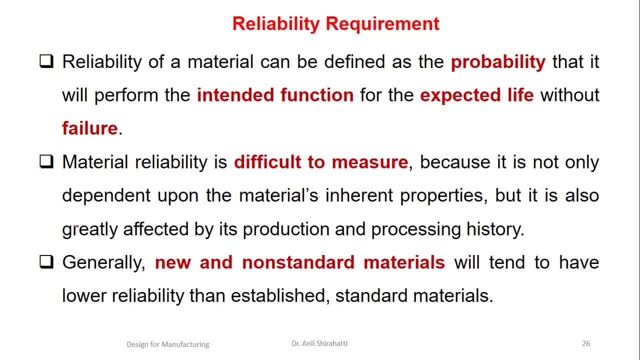 is there. that is the testing with respect to time at either room temperature or high temperature. this test will give an idea of reliability of that material with respect to time. but if you see the testing time, it will go from one month till five, five, six, six years of continuous testing. 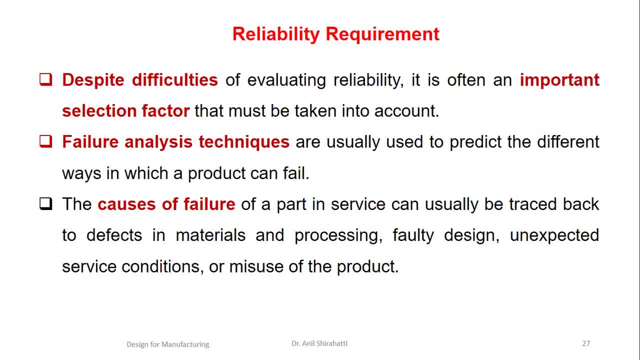 despite difficulties of evaluating the reliability, it is often important selection factor that must be taken into account. failure analysis techniques are usually used to predict the different ways in which a product can fail. the cause of a failure of a part in service can be usually be traced back to defect in material process, faulty design, unexpected service condition. 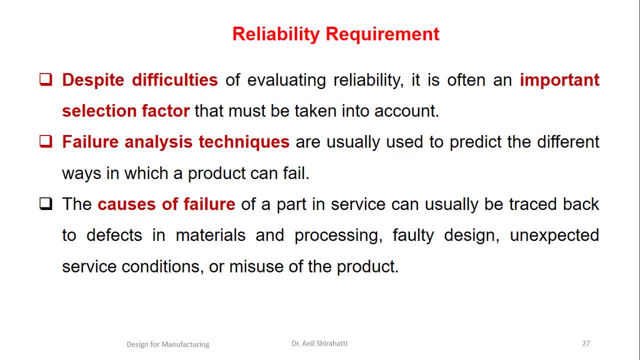 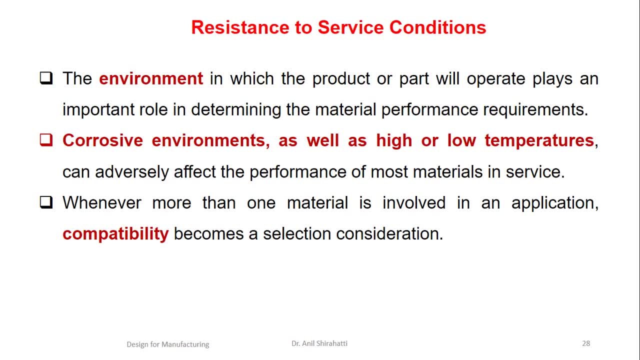 or message of the product when i am doing any reliability requirement tests. the last one is resistance to service condition. the environment in which the product or part will operate plays an important role in determining the material performance requirement. corrosive environment as well as high or low temperature are adversely. 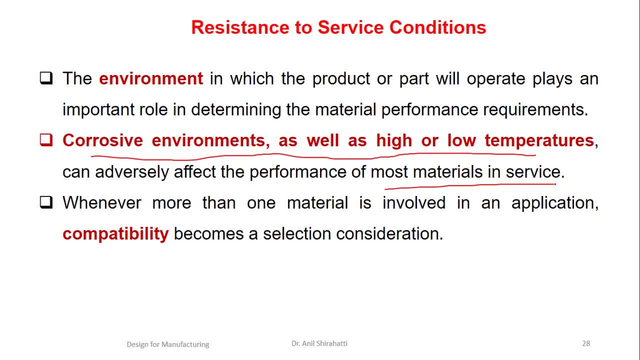 effective material performance in service. whenever more than one material are involved in application, compatibility becomes a selection consideration. for example, if the temperature is, let's say, 250, i have to go for mild steel, or, and let's say stainless steel, i may not go for a plastic. 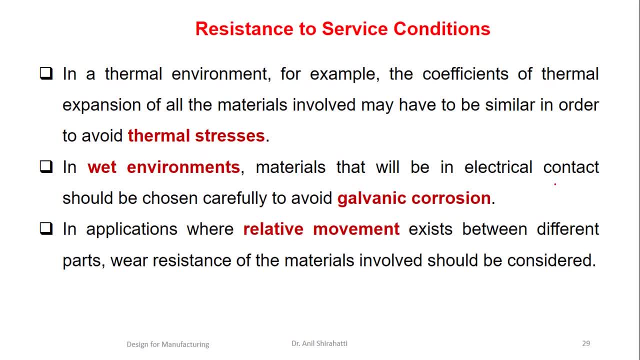 in that case, in thermal environment, for example, the coefficient of thermal expansion of all the materials involving may have to be similar in order to avoid any thermal expansion or thermal stresses. in wet environment, material that will be in electrical contact should be chosen carefully to avoid any galvanic corrosion effect in application where relative movement exists.